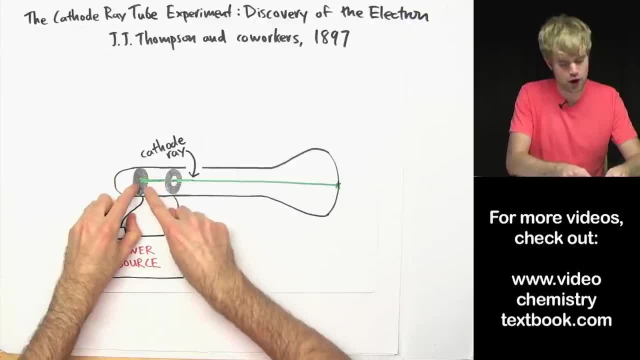 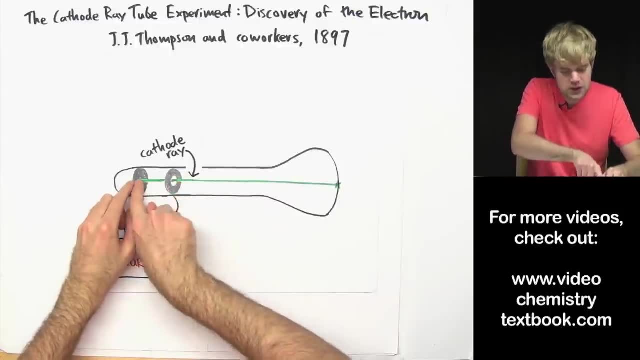 But what really was going on is that electrons from this piece of metal were shooting out. They were attracted to this piece of metal, which has an opposite charge, but they were moving so fast that they shot all the way across the length of the tube. 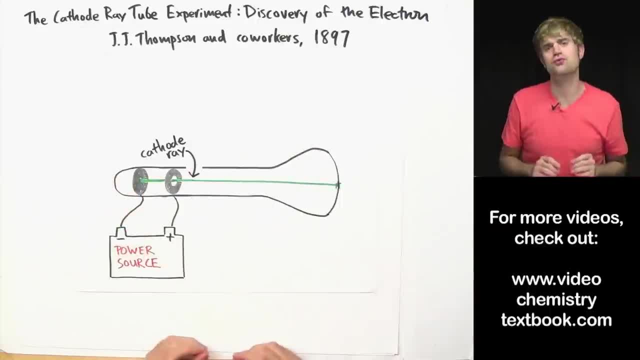 Anyway, Thompson sees this ray and he gets curious as to what it's made of, And so he asks the question: the stuff that the cathode ray is made of, does it have an electrical charge? And here's how he attempts to answer that question. 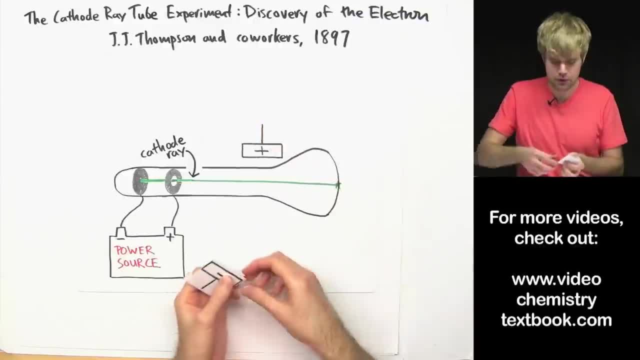 He takes two metal plates and puts them on either side of the cathode ray tube And then he turns on electricity, which makes the top plate positively charged and the bottom plate negatively charged, And check out what happens to the cathode ray When he turns on the power. 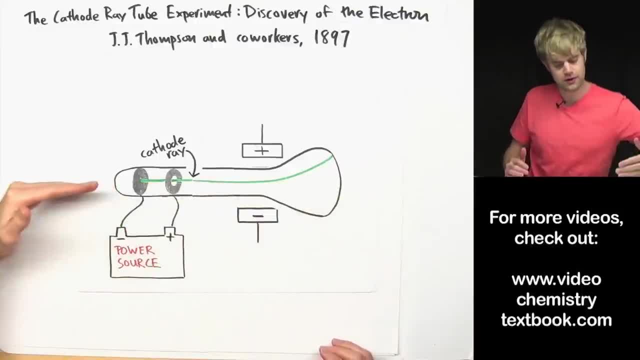 he sees that now, instead of going straight through, the cathode ray bends up. It bends up towards the positively charged plate. So, based on this, he reasons that the cathode ray must be made of stuff that's negatively charged, since it's attracted to the positively charged piece of metal. 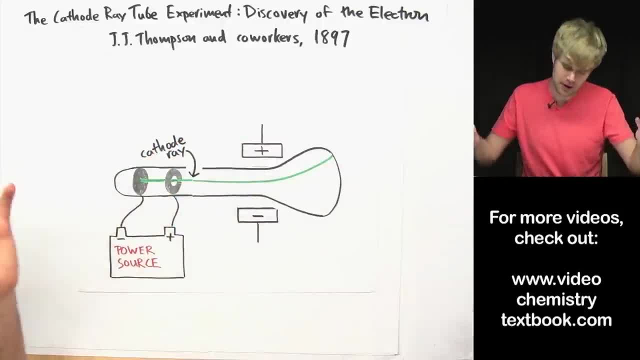 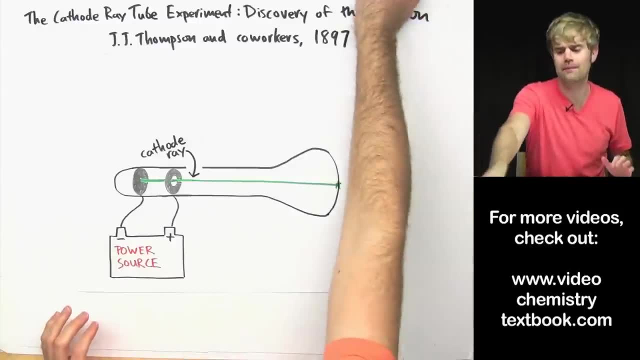 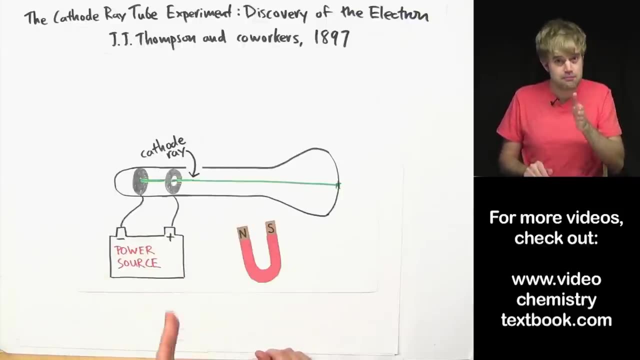 and he knows that opposite charges attract. But just because he wants to be very careful- he's a very careful guy- he tries to check this another way, So he uses a magnet. If something has an electrical charge and it's moving, a magnet will push it in particular directions. 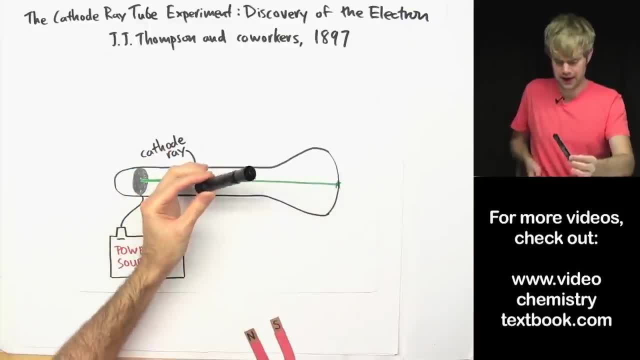 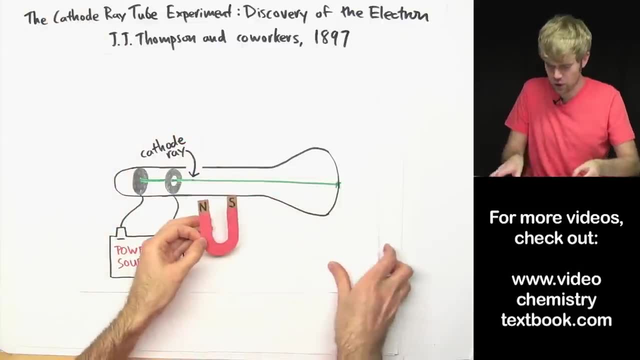 So he takes a cathode ray tube- if you want to think that this marker is kind of the cathode ray tube- and he surrounds it with a magnet, just like this. We can kind of show what goes on by slipping the magnet under, like this: 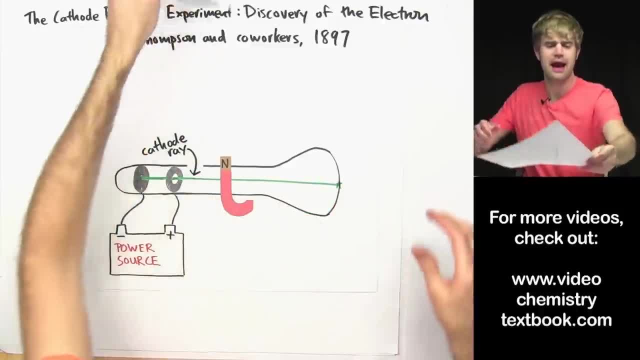 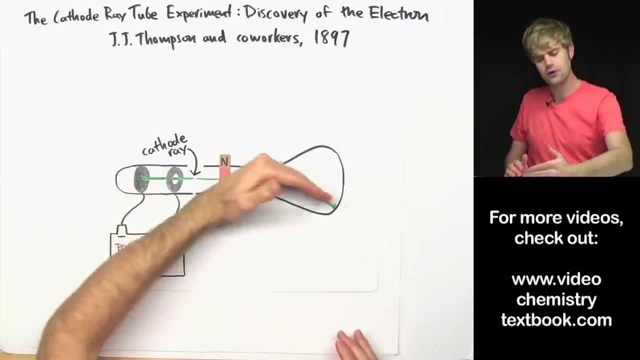 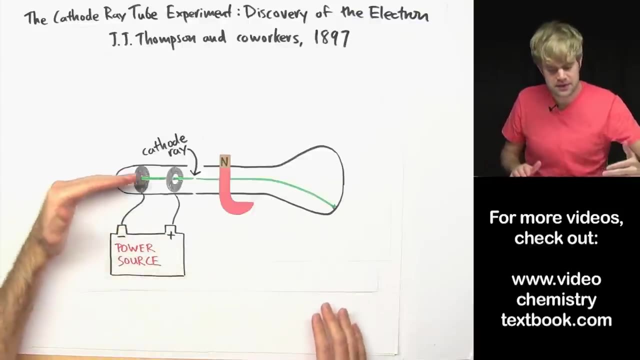 So, anyway, he puts the magnet here and he sees now that the cathode ray bends in the other direction, It now moves downward. Now, if the cathode ray is indeed negatively charged, this is exactly how he would expect it to move in the presence of a magnet like this. 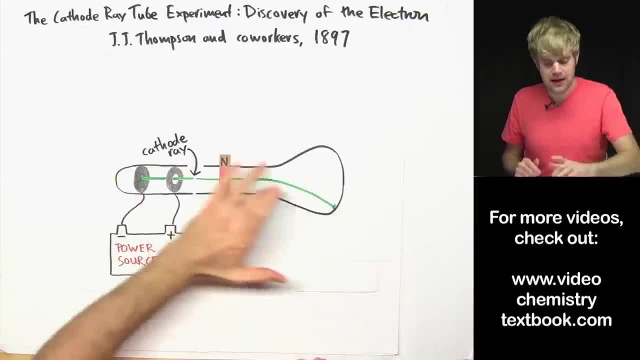 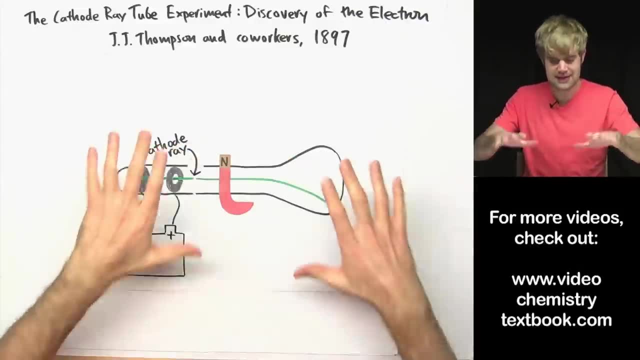 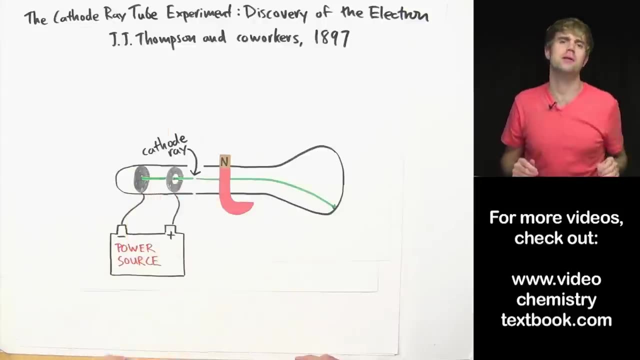 So this is just further confirmation that whatever makes up the cathode ray probably is negatively charged. So he takes the data that he gets from these experiments and he's able to draw a few important conclusions about cathode rays and what makes up atoms. Okay, so, based on the outcomes, 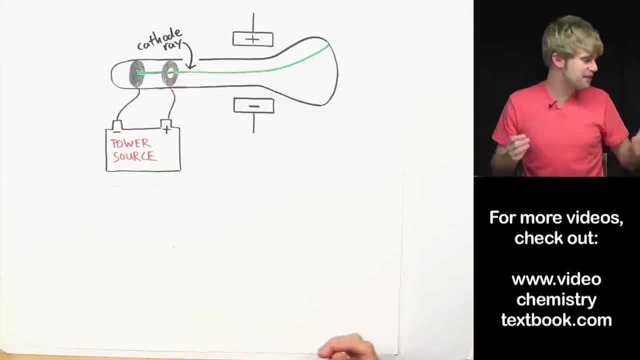 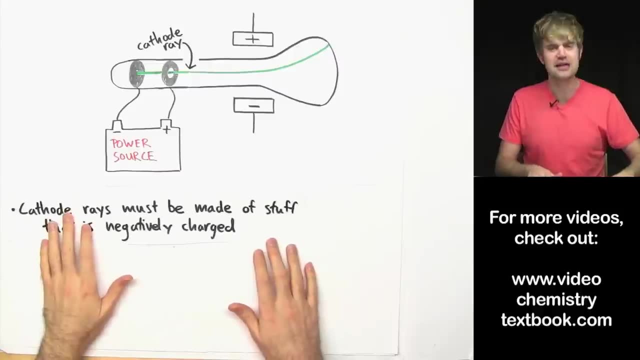 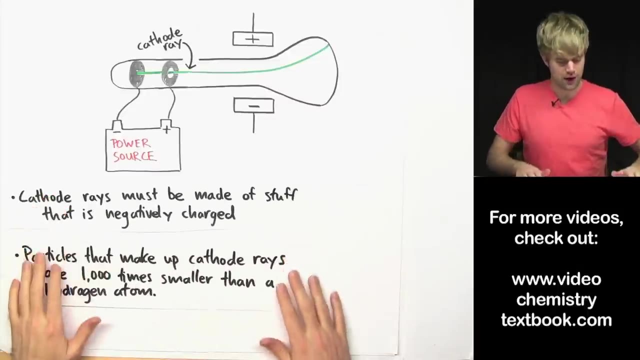 of the experiments with the charge plates and the magnet, Thomson is able to conclude that cathode rays must be made of stuff that is negatively charged. He combines the information that he got from the experiments that I just told you about with some other data that he collected. 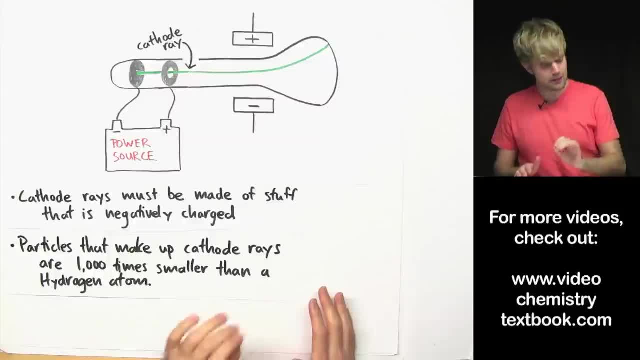 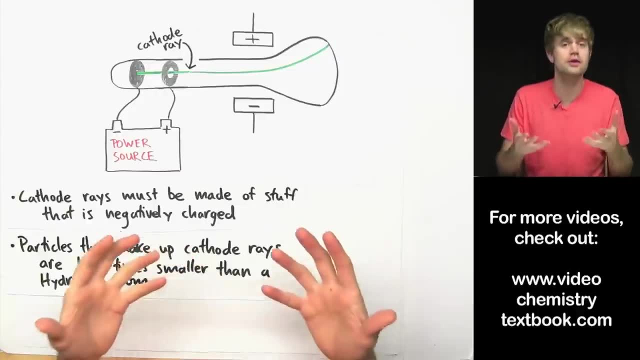 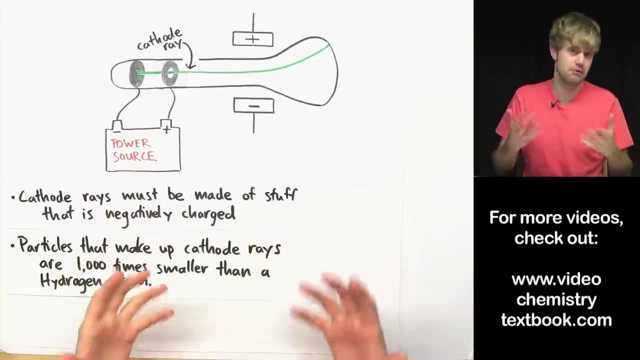 and he's able to come to the conclusion that the particles that make up cathode rays are a thousand times smaller than a hydrogen atom. Hydrogen atoms are the smallest atoms, So this thing that's in the cathode rays must be really, really tiny compared to an atom. 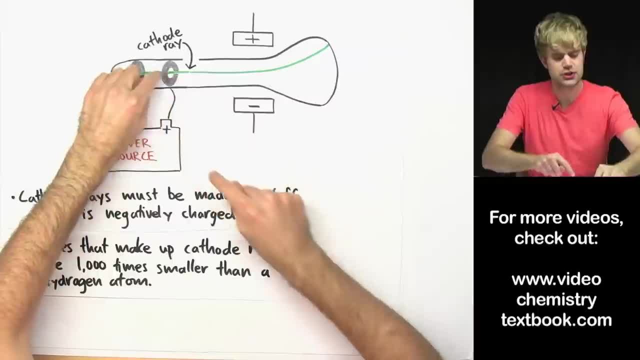 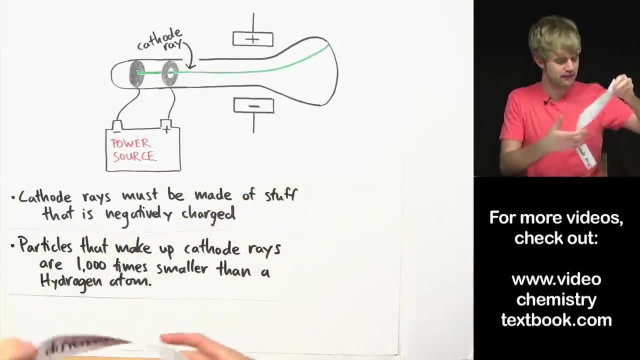 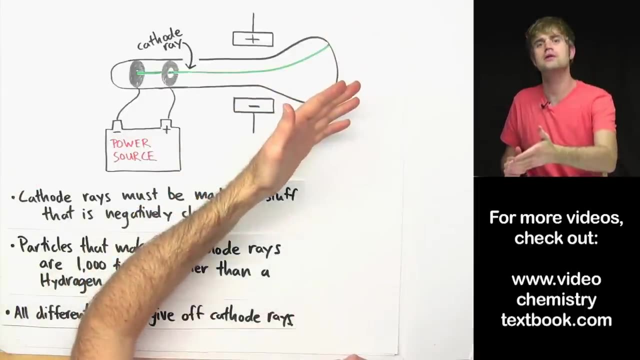 And finally, Thomson swaps out the type of metal that's in the cathode tube. He uses a variety of different types of metal, but he finds that all of the different metals he uses give off the same cathode rays and regardless of what metal he uses. 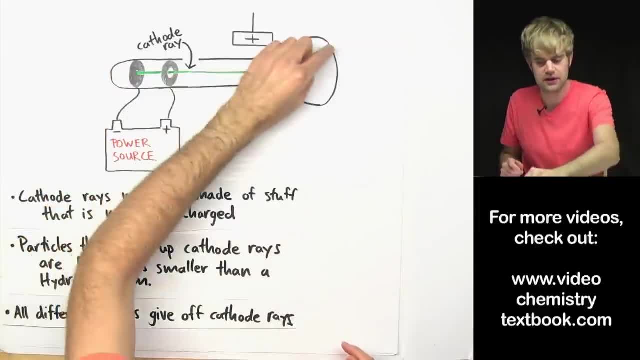 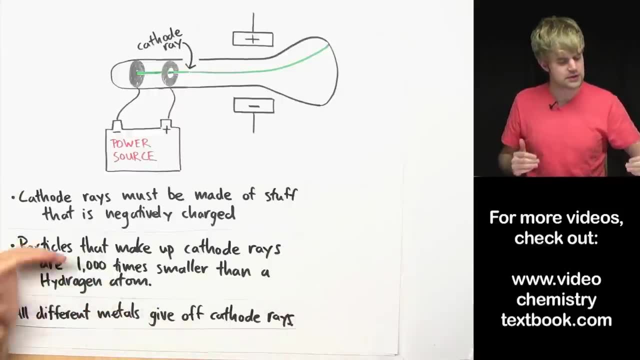 the size of the things that are in the cathode rays is exactly the same. So, based on these three conclusions, he's able to come up with the idea that atoms have tiny negatively charged particles inside them and these things that we're talking about here. 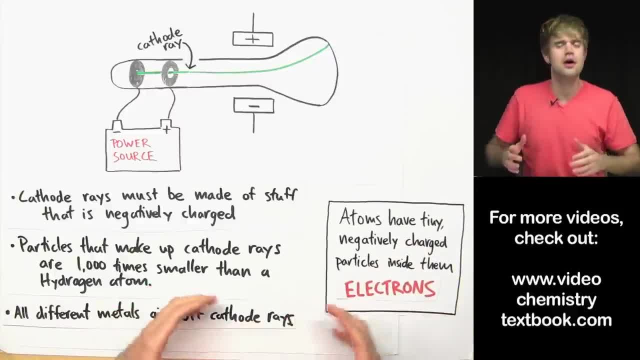 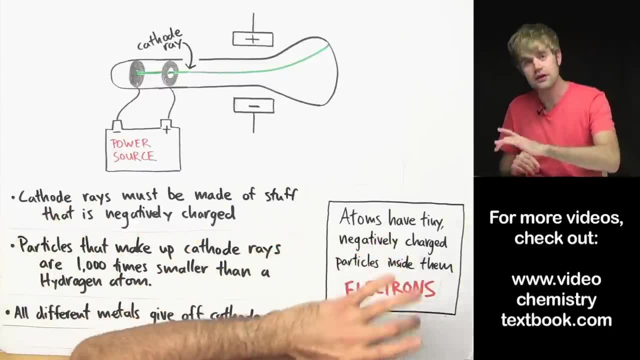 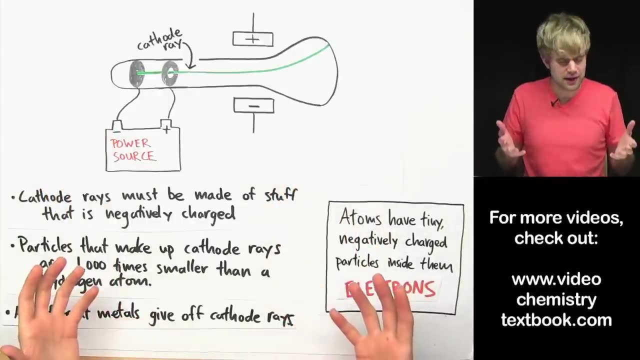 are electrons. Now, if you're like me when I first learned this, you might be confused how these conclusions definitely tell him that there are electrons inside atoms. I remember when I first learned this stuff I was thinking like wait, doesn't this just show that electricity? 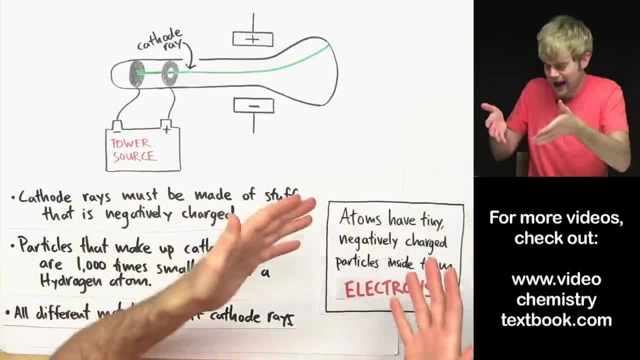 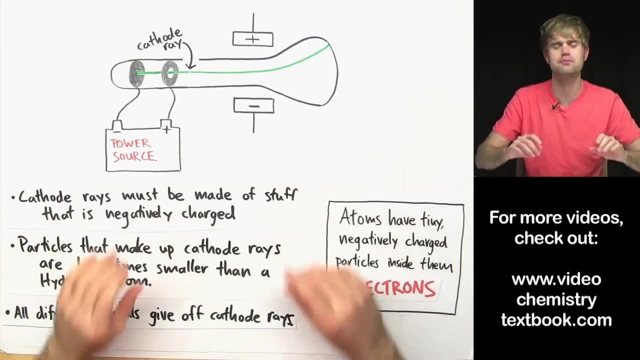 or cathode rays have negatively charged stuff. How does this tell us anything about the atoms? Okay, here's why, At the time that Thomson does his experiment, everyone for the most part agrees that all things are made up of atoms. 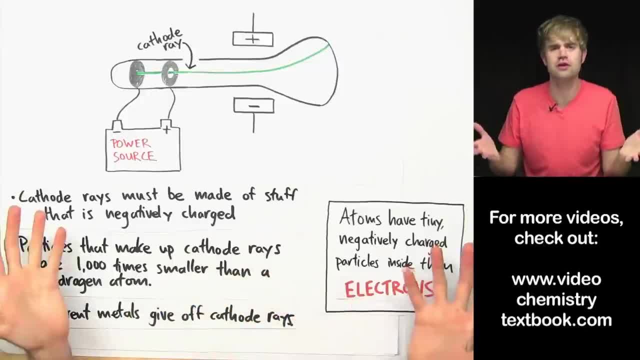 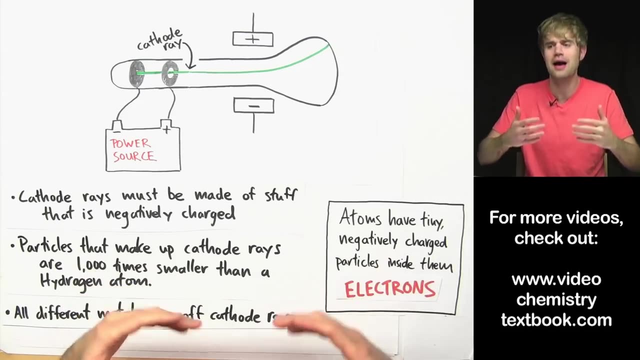 that atoms are the smallest things that make everything up. They're like the smallest things in the universe. So if Thomson is able to show that there are even tinier things, well, where are those tiny things coming from? They have to be coming from atoms. 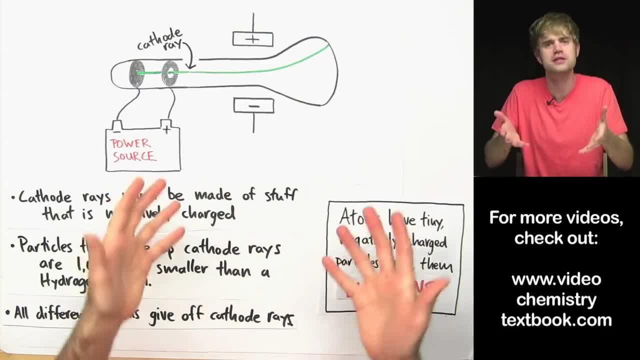 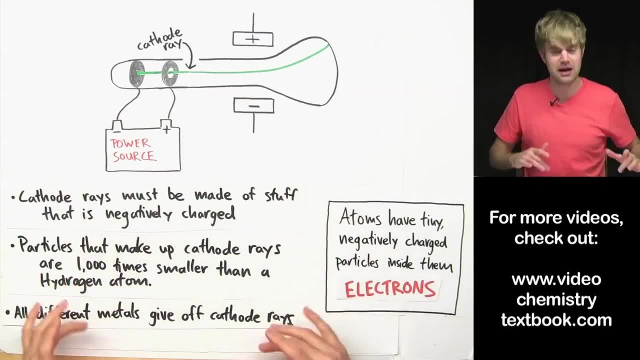 because everything's made of atoms, right, That's the only place they can be coming from. And even if electricity, even if you want to say that you know, oh well, he's just showing that electricity is made of electrons. 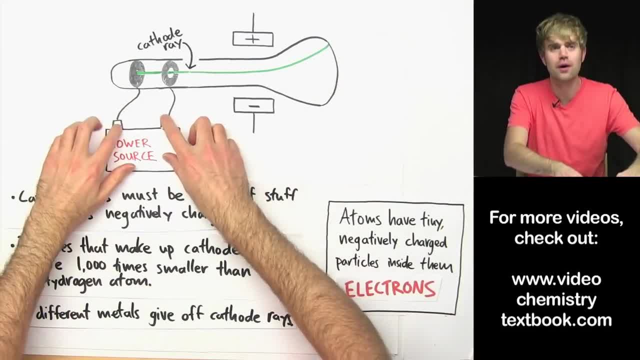 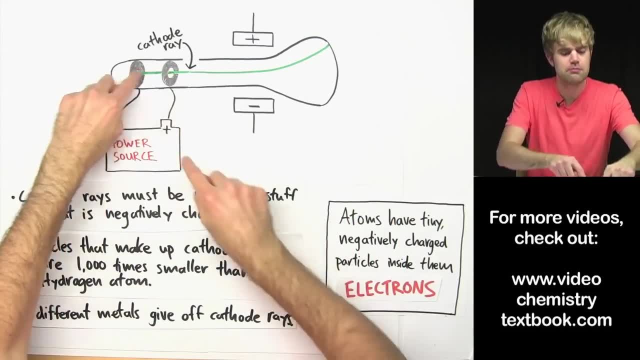 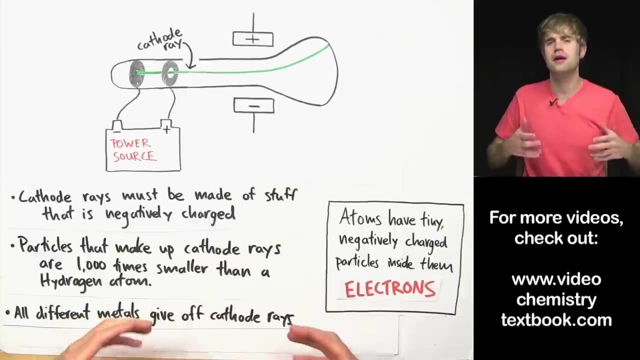 well then still, where are the electrons coming from that make the electricity? The electrons have to be coming from other atoms. And since he can move and remove these pieces of metal and swap other metals in and he still gets electrons, it again shows that all different types of atoms 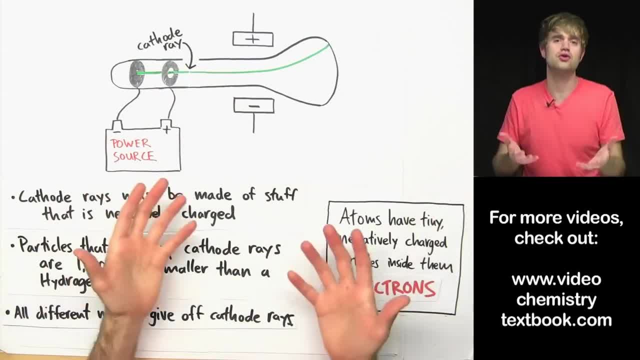 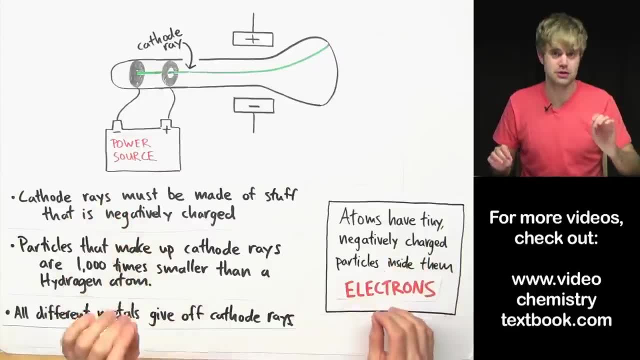 are able to release or give off electrons, So they must be in there to begin with. Anyway, these conclusions that Thomson comes to have dramatic effects on how scientists think about what the atom actually looks like. Now, at the beginning of the video, 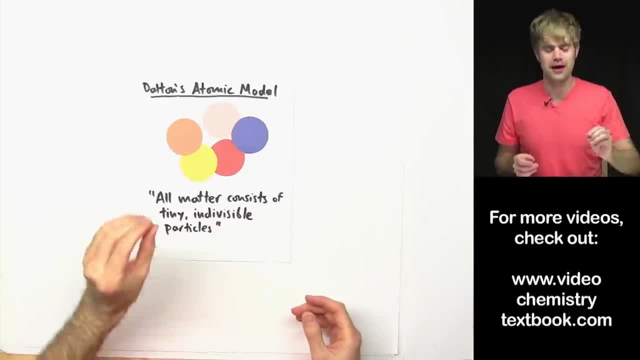 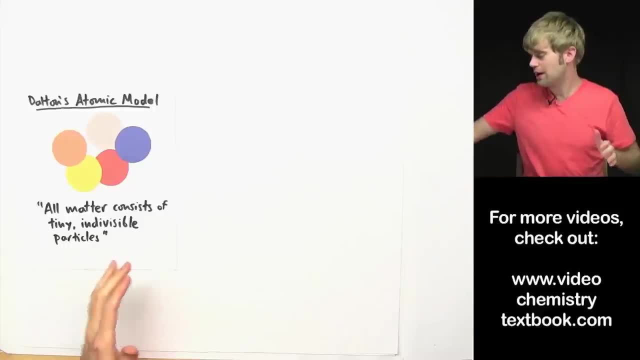 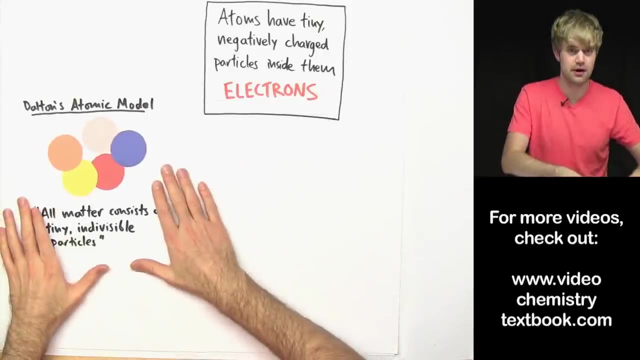 we said that in Dalton's atomic model atoms are indivisible, that they're not made of anything smaller. But when Thomson discovered that atoms have tiny negatively charged electrons inside them, he essentially disproved this model, at least the part about the indivisible atoms. 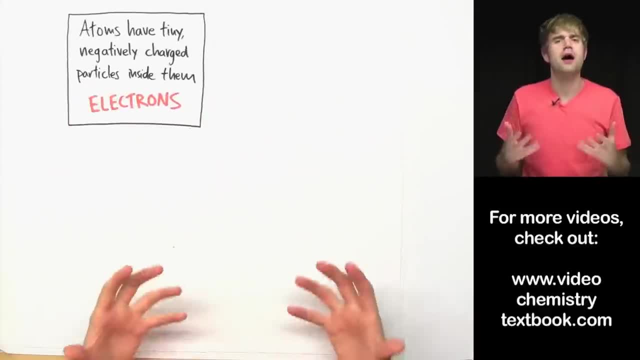 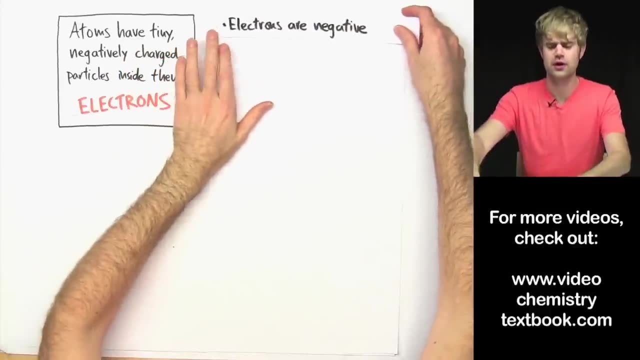 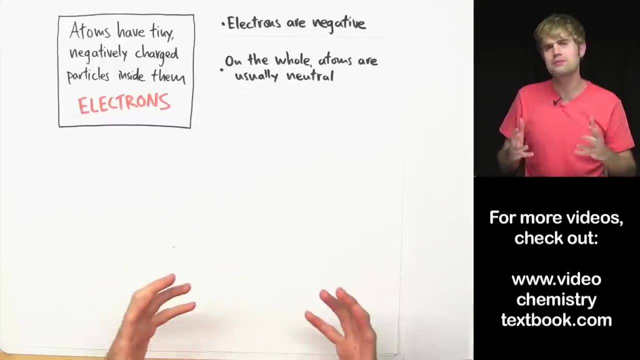 So here is the model of the atom that Thomson comes up with. He realizes first of all that electrons are negative- We already talked about that- But then he notices that on the whole, atoms in general are usually electrically neutral. 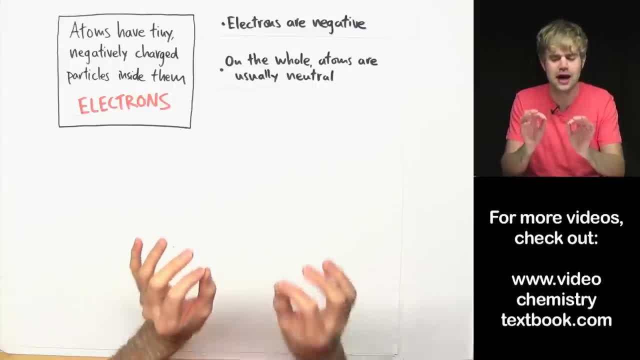 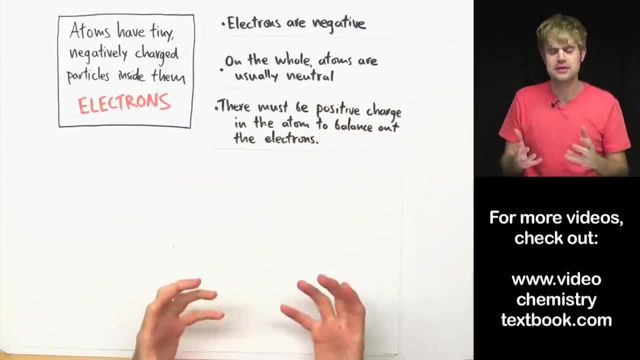 So even though they have these negatively charged electrons inside them, the atoms as a whole don't have a charge. So Thomson realizes that in order for the atoms not to have a charge, there must be some positive charge in the atom that can balance out. 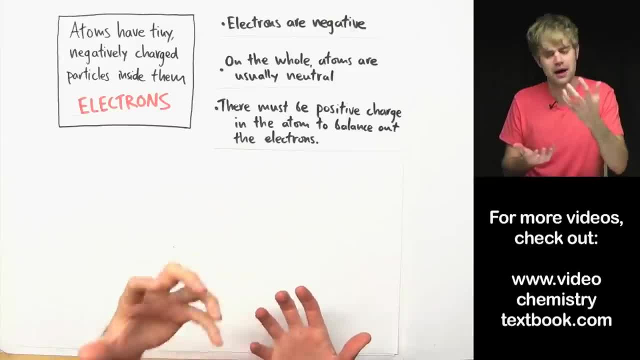 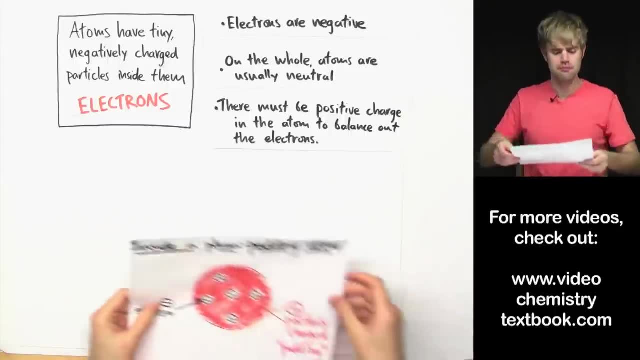 the negative charge of the electrons And then the positive and the negative balance out and the atom then as a whole doesn't have a charge. So he comes up with a model that he calls the plum pudding atom. Now, plum pudding is kind of a British thing.